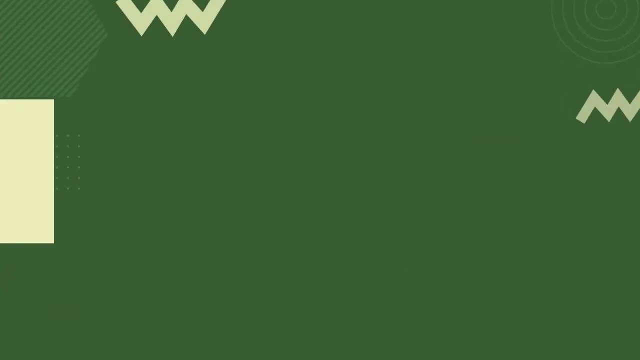 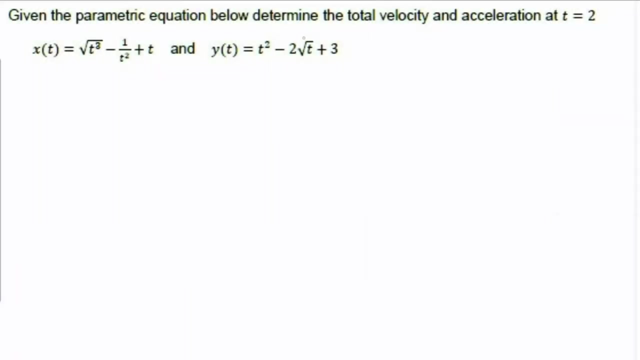 We are given the parametric equation below and we are given the total velocity and acceleration at equal to 2.. So, first off, there are two components. One is the x, when the velocity will be in the x component, since there is a displacement in the x component and towards 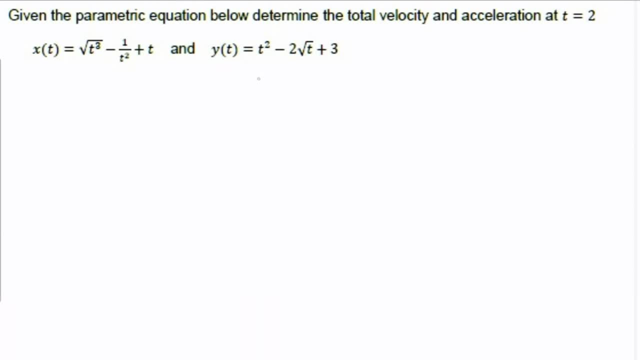 the y component as well, and same is applicable for acceleration. So let's first talk about velocity. Velocity in the x component will be x prime x prime t. So that's going to be a d over dt of cube. square root of t cube can be written as t raised to 3 over 2.. 1. 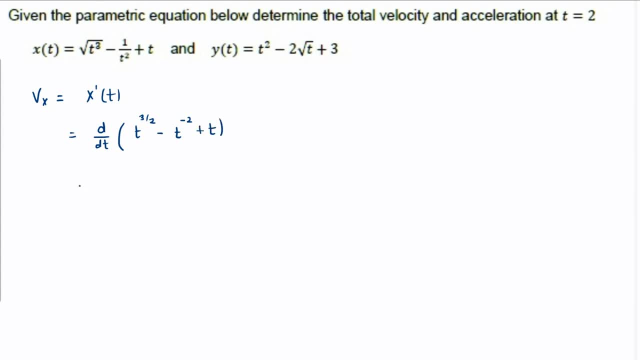 over t square can be written as t raised to minus 2 and this plus t, So this will become 3 over 2. times t raised to 1 over 2 minus minus 2 comes down. This will become t raised to minus 3 and this is plus 1.. So this will become 3 over 2 root. 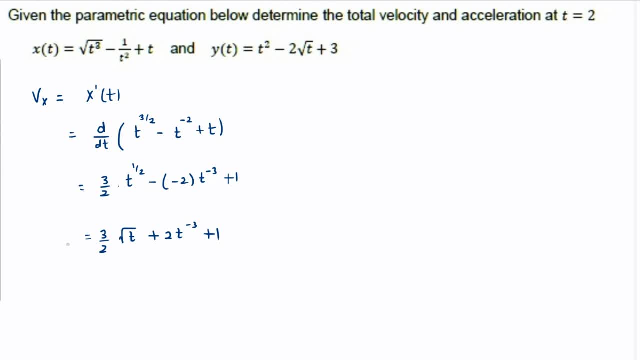 t plus 2, t raised to minus 3 plus 1.. So, at t equal to 2, what is the value? At t equal to 2, px at 2 is 3 over 2 times root 2 plus 2 times 2 raised to minus 3 plus 1.. So this: 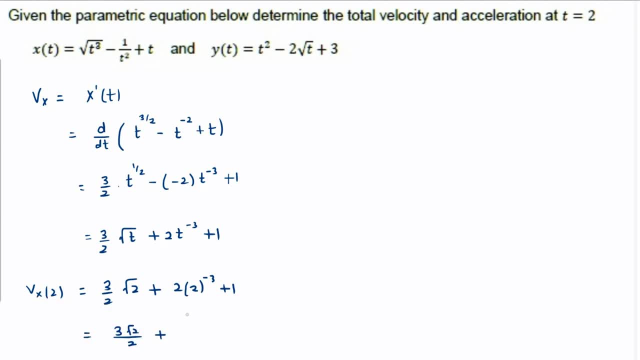 will become 3 root. 2 over 2 plus 2 over 2 cube is nothing, but 1 over 2 cube is 8.. So 2 over 8 is 1 over 4 and this is plus 1.. So this is the velocity, the x component. 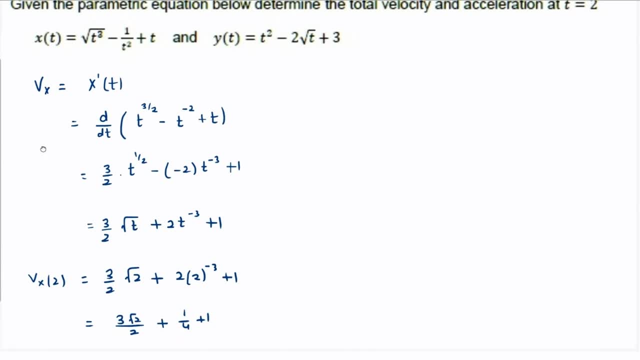 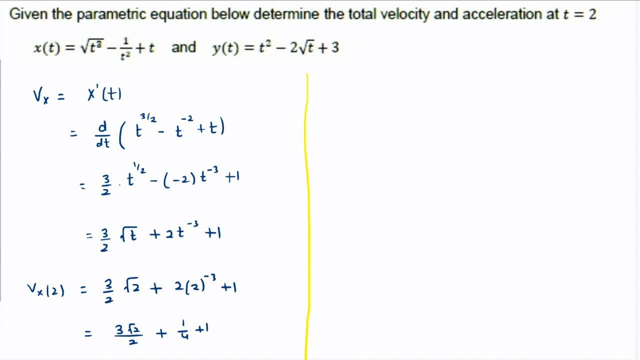 The velocity. I'm not sure if they're interested in this, because this is the exact value they're interested in in the net value anyway. So let's find Vy likewise. So Vy is going to be y prime t, So y prime t is going to be 2t minus 2 times 1 over, 2 times t raised to. 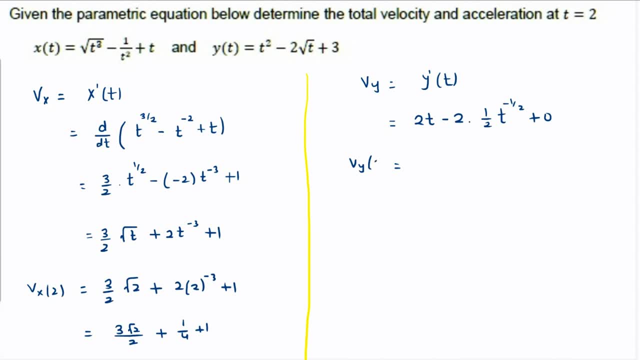 minus 1 over 2 plus 0. So Vy at t equal to 2 will be 4.. And these two are cancelled, Minus 2 raised to minus 1 over 2.. So this will become 4 minus 1 over root 2.. This is: 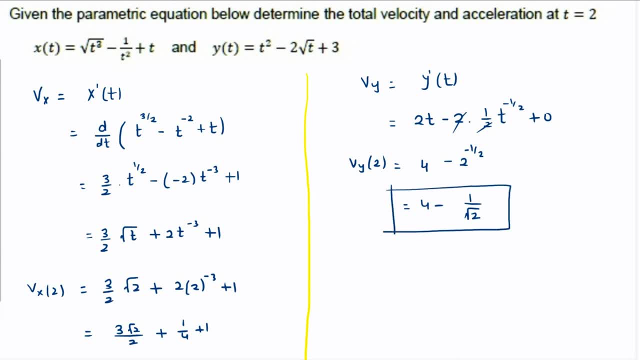 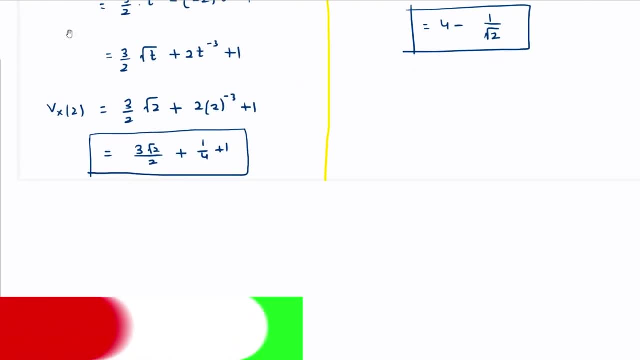 the value of Vy at t equal to 2.. And we have Vx, we have Vy, So the net velocity is definitely the vector sum of these. And since these are the two vectors, x is over here, y is over here, So these are at 90 degree. So net velocity is going to be square root of Vx. 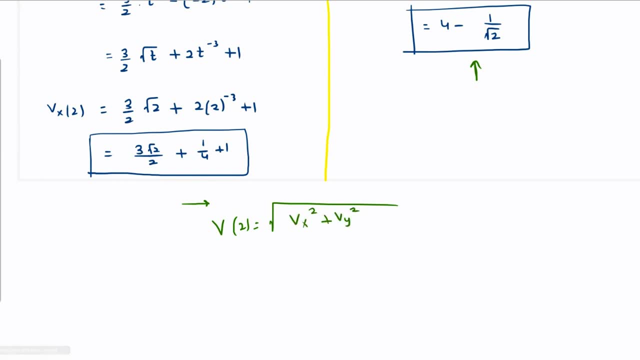 Square plus Vy square. So all we have to do is a square of this and a square of this as well. So that's where the calculator comes in. Just grab my calculator. This would be 3 root 2 over 2 plus this value, square of this value plus uh plus 4 over 2.. So that's. 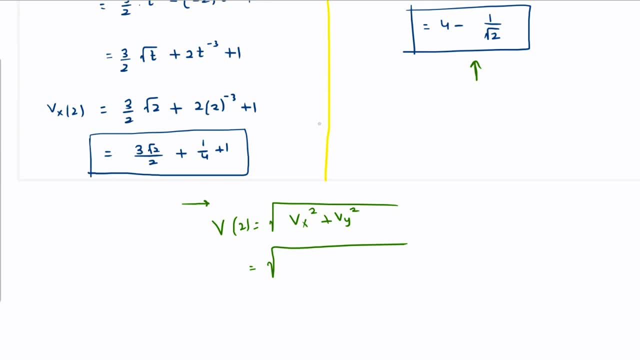 4 minus 1 over root, 2 square, And the square root of this value comes out as 4.71.. 4.71.. And the unit will be: uh, there's no unit given, So I'll just write the absolute number. 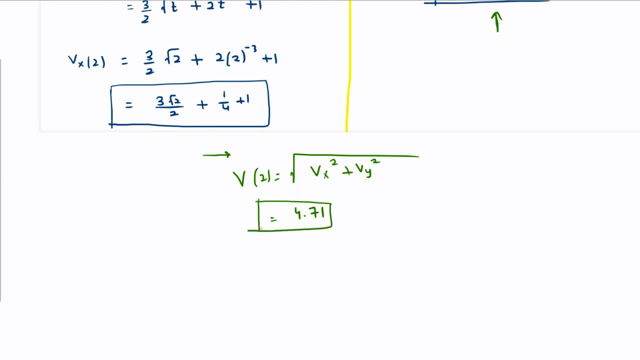 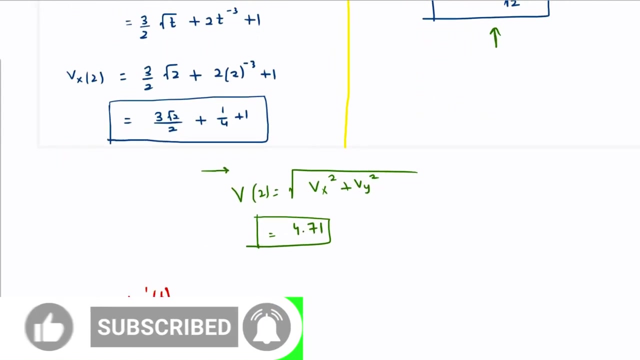 without the unit. So it's 4.71.. Uh, likewise, now I'm going to work for acceleration. So the acceleration towards x side will be V prime x, V prime sub x. So what is V prime x, which is this? So we just have to differentiate. 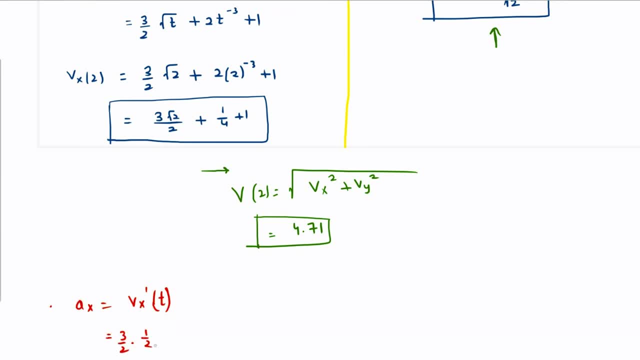 this once again. So this will be 3 over 2. remains as it is, This will become 1 over 2 times t, raised to minus 1 over 2.. And this will become minus 3 times t, raised to minus 4 plus 0.. 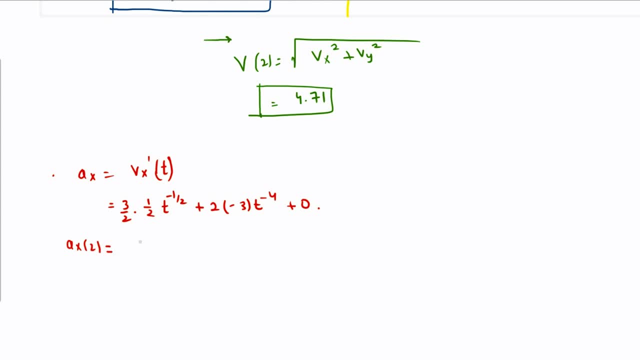 So the value of acceleration at t equal to 2 will be uh 3 over 4 root t And where is nothing but 2.. So 2 and then minus 6 over minus 6 over t raised to 4, where t is 2 and 2. 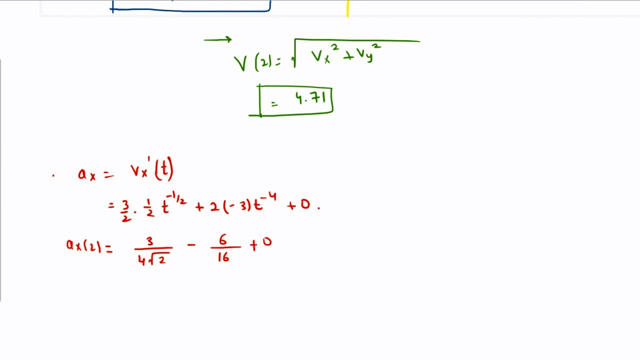 raised to 4 is 16, and this is plus 0. So this will become- let's keep it as it is. I mean, this can definitely be simplified- 2 is a common factor, So this will become 3 over 8.. So this is the. 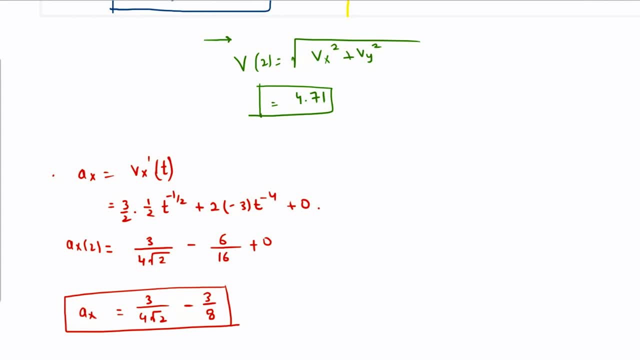 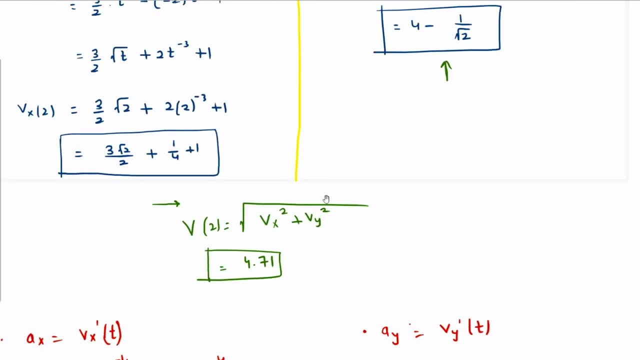 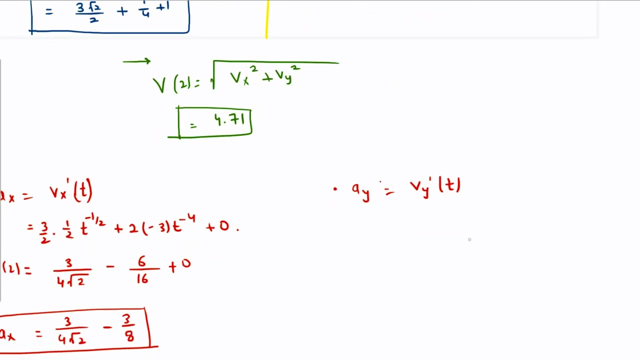 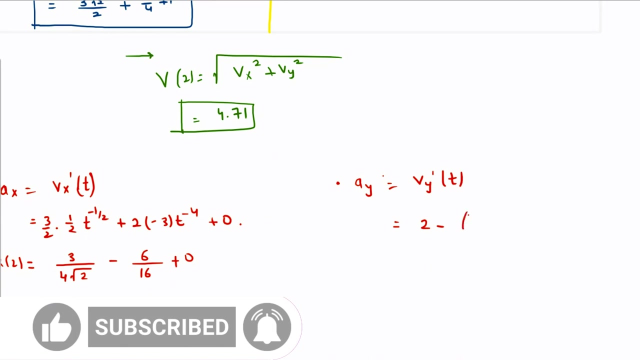 acceleration towards the x direction and likewise towards the y direction. it's going to be v prime t of v y prime t. So this v y- it is over here- 2 t minus 1 over root t. So this will become 2 minus, and that was t raised to, minus 1 over 2.. So this will be minus 1 over 2 times t raised to. 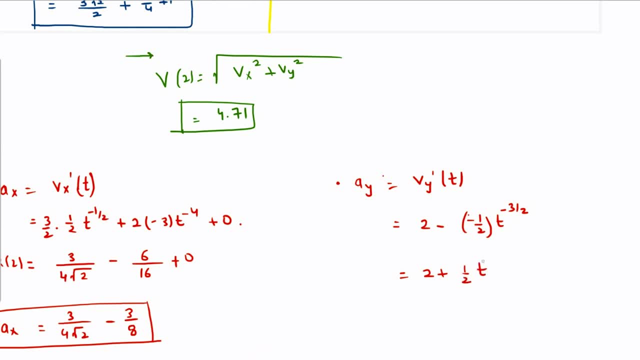 minus 3 over 2.. So this will become 2 plus 1 over 2 times t, raised to minus 3 over 2.. This is a y, So the value of a y at 2 is going to be 2 plus 1 over 2 times 2, raised to minus 3 over 2.. So we got both a x and a y. So 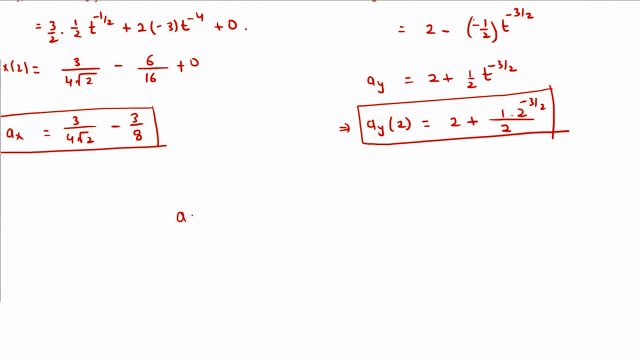 the net value of the acceleration is going to be just like the velocity. It will be a x square plus a y square. So that's going to be- let me just grab my calculator. That will be 3 over 4 over root 2.. 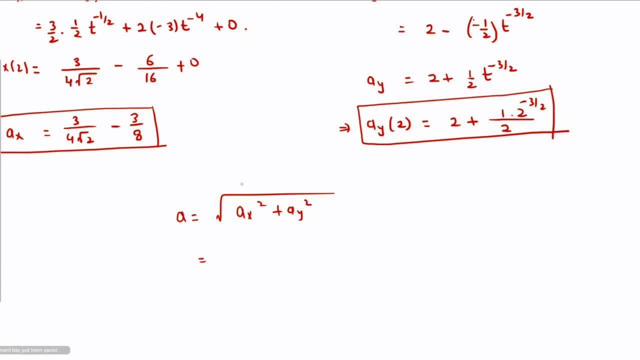 minus 3 over 8 square of this value. plus 2 plus Become 4 over 2, 1 over 4 over 2, 15 say 3 over 4 versus two square root of this value. but that will be a 2.4 square over this value. 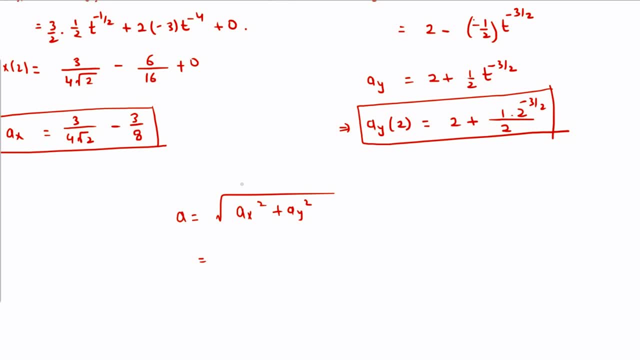 slash negative 0 with this square root of this value. let's show this move the lambda be a th. Thank you, brother. temos 2 superview: We gonna add. Did you get it? Press the f button unless you do.